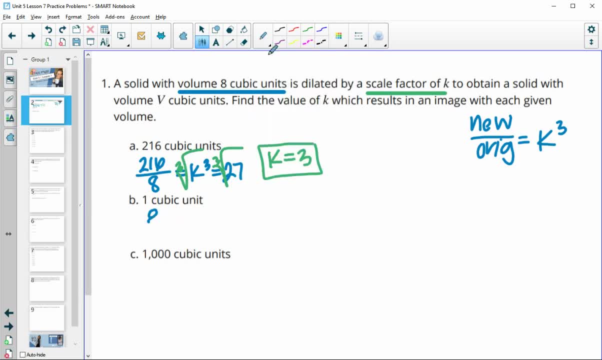 For this next one we had a volume whoops- a new volume of 1 and an original volume of 8, so 1 over 8 is our k cubed value. So then we will cube root each of these and get that k cubed is 1 half. 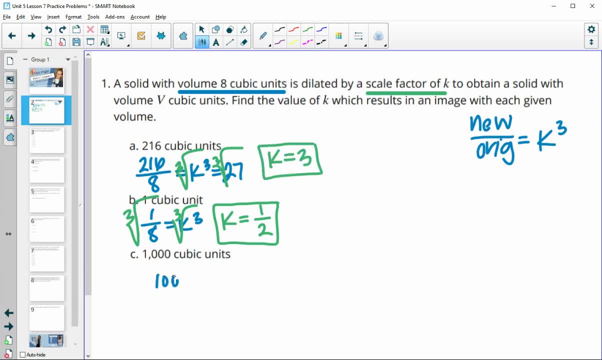 And then this third one. our new volume is 1,000, our original volume was 8,. again, that's our k cubed, and both of those are perfect cubes, so we could just cube that right away. do the cube root? 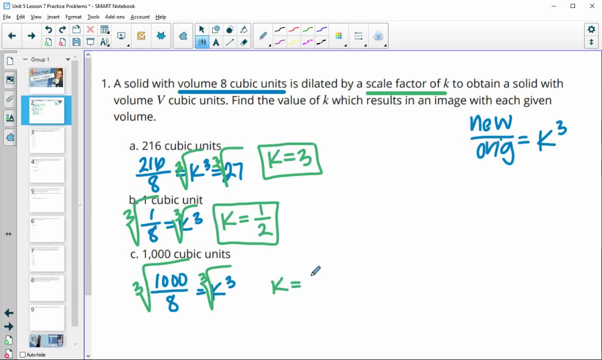 of that right away. Once again, we have the atty ratio, but we're going to weigh my job right now and our sum could be compounded by that and we could alsoww, we could echo out the old number, But um, but this half it's now basically. 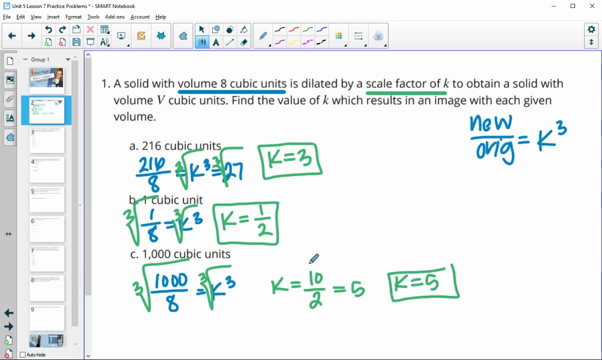 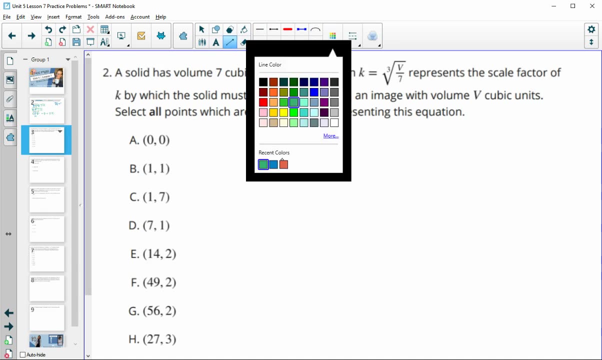 equal to the atty ratio. so then we're going to 123.. So we've got that product right now. And then what we're going to do next? we are going to want to��mlt multiple of this, and that's going to tell us that our k is equal to 10 over 2, which then simplifies to 5.. And if you had just divided right away 1000 divided by 8, wouldow have been 125, and then the cube of that is 5.. Number 2, solid, has a volume of 7 cubic units, and then we've got this equation here. we would loss out 276 minus. 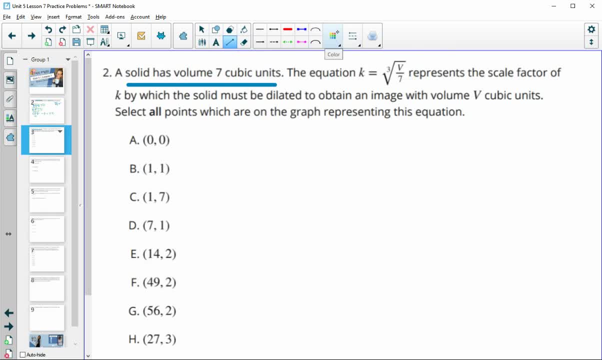 8 cc, this equation here that represents the scale factor by which a solid must be dilated to obtain the new volume. select all the points that are on the graph of this equation. So K is our output or our Y value. Okay, So this is going to be our second value, And then our V is what's being? 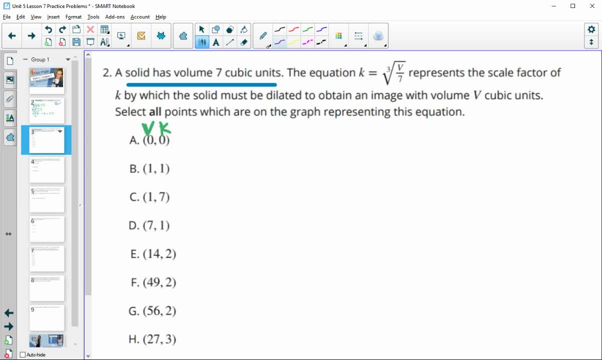 plugged in. So we're going to plug in this first number, okay, into this cube root, and see if it equals out to this second number. So we will do the cube root and then I'm just going to write it horizontally here, of V, which is zero divided by seven. So the cube root: zero divided by seven. 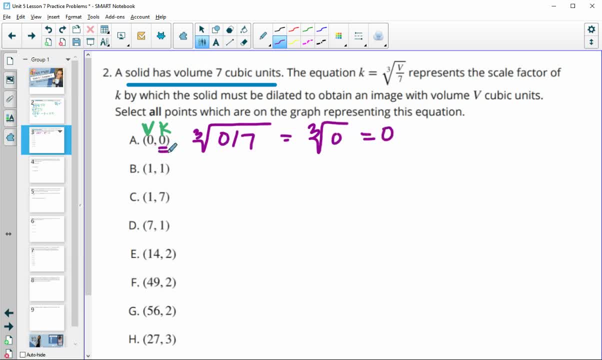 is zero, The cube root of zero is zero, which does match this. So when we plug in zero, we get back zero, which is that ordered pair. Next one: we will plug in the one. So we'll do the cube root of one divided by seven, and that is not going to equal one. So that's just going. 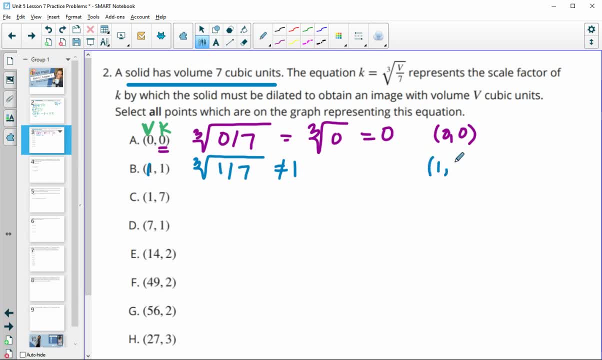 to be the cube root of one seventh. So if we plug in one we get back the cube root of one seventh, which is not what we have here, So that one does not work. Next one, So we'll plug in one, And so then we get the cube root of one over seven again, And 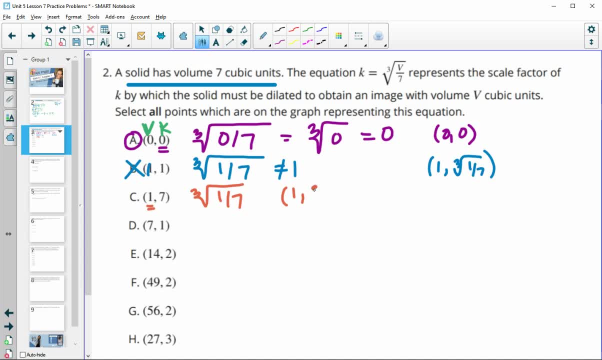 that doesn't simplify. So when we plug in one, we get back the cube root of one seventh, which is not what this says. So this is not good. Next one. So we will plug in seven. So the cube root of seven divided by seven and seven divided by seven is one and the cube root 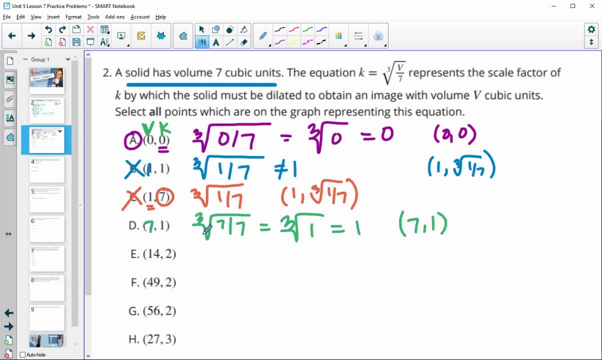 of one is one. So when we plug in seven we get back one, which is this ordered pair. Next one we'll plug in 14.. So 14 divided by seven is two, and the cube root of two is not a nice. 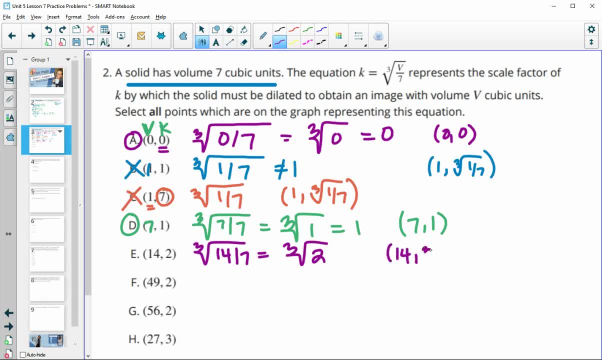 number. So it'll just stay like this. So when we plug in 14, we get back cube root of two. So that is not correct. where that point is not on the graph, Next one, we'll plug in 49.. So 49 divided by seven and then the cube root of that. 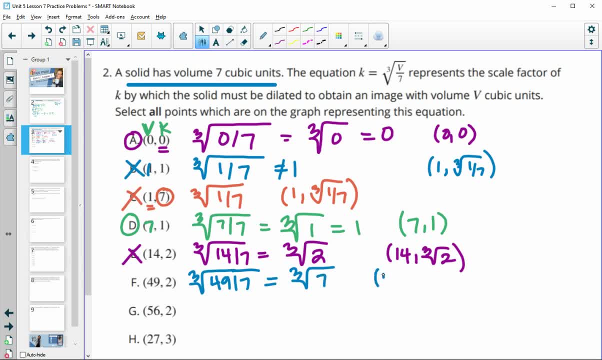 49 divided by seven is seven. So when we plug in 49, we get back the cube root of seven, which is not two, So that one is not correct. Next one we will plug in 15.. 56. And 56 divided by 7 is 8. And the cube root of 8 is 2.. So when we plug in 56, we get back 2.. 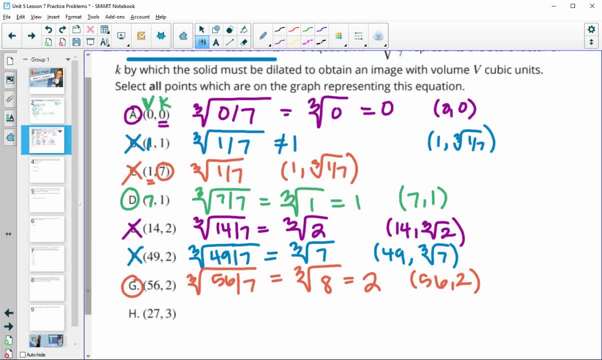 And that's what this said. So this point is on the graph, And then the last one. for this one we'll plug in 27.. So we have 27 divided by 7.. And 27 divided by 7 is not nice. So when we plug, 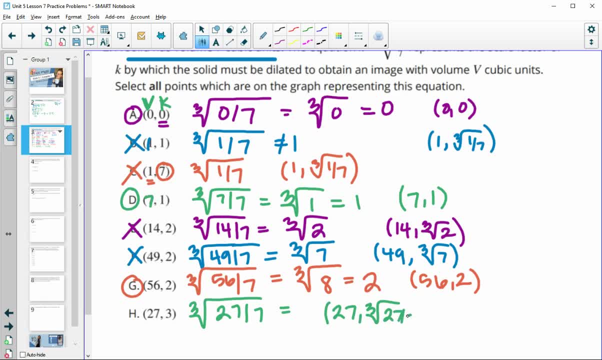 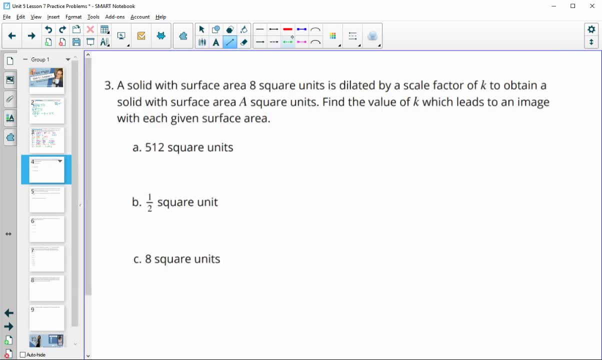 in 27,. we just get back the cube root of 27 over 7, which is not this ordered pair. Number three: a solid with a surface area of 8 square units is dilated by a scale factor of k to obtain: 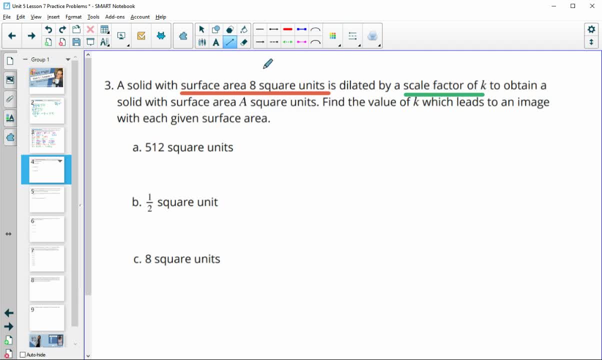 These surface areas below find the value of k that leads to this surface area. So remember, when we're dealing with areas, we are dealing with k squared. So when we take our new area divided by our original area, we are going to get back k squared, And so 512 divided by 8. 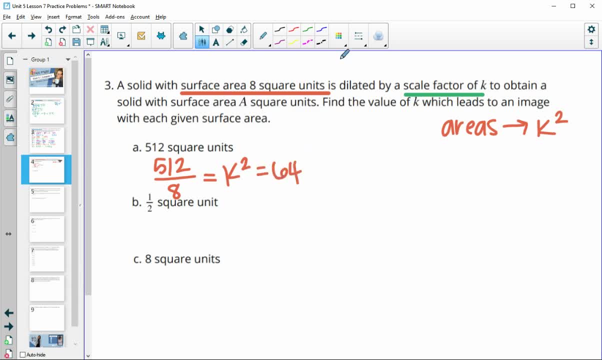 gives us our k squared, which is 65.. So then, to get down to the scale factor, we'd have to square root, And we get k equals 8 in this one. Next one: our new area is 1 half, And our original area was 8.. This is our k squared. 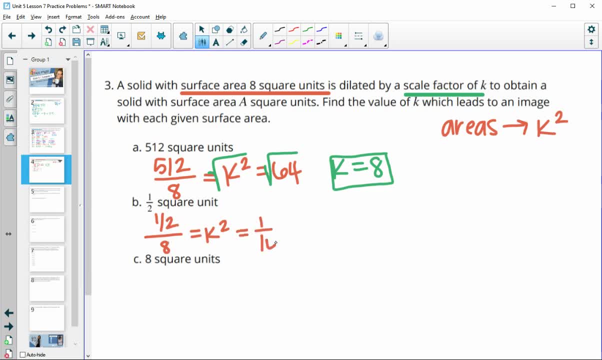 And so 1 half divided by 8 is 1: 16th. Then to get k, we would square root both of these. And so the square root of 1 is 1: 16th. And then to get k, we would square root both of these. 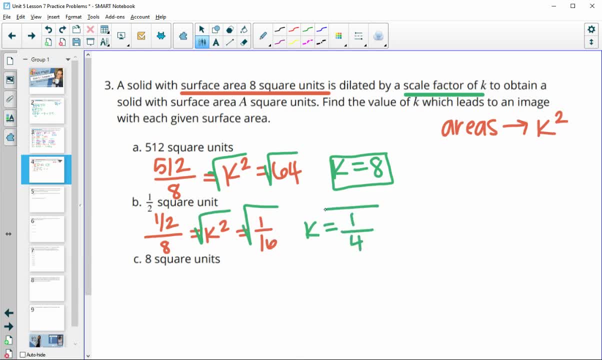 1 for the top is just 1. And the square root of 16 for the bottom is 4.. So the scale factor is 1, 4th And then this final one. our original area was 8. And our new area is 8. So then you can do. 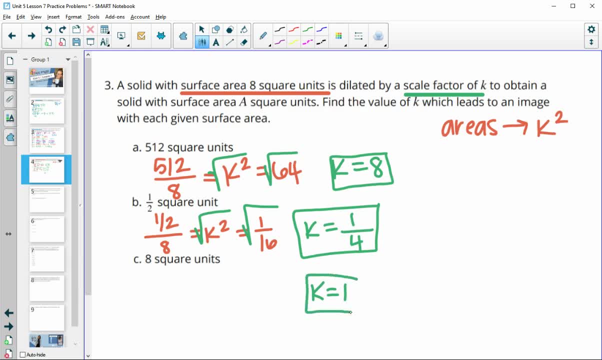 the work Or you can recognize that nothing changed. So the scale factor is 1.. But if you wanted to go through the process you would do: the new 8 divided by the original 8 is your k squared, which is 1.. And then square root. 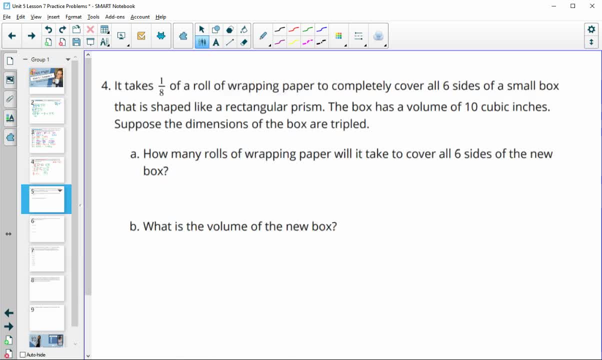 All right. number four: it takes 1 eighth of a roll of wrapping paper to completely cover all six sides of a box. So when we're talking about wrapping paper, that's going to be an area idea, So this is an area, And then we don't really care how many sides of the box is, just how much it. 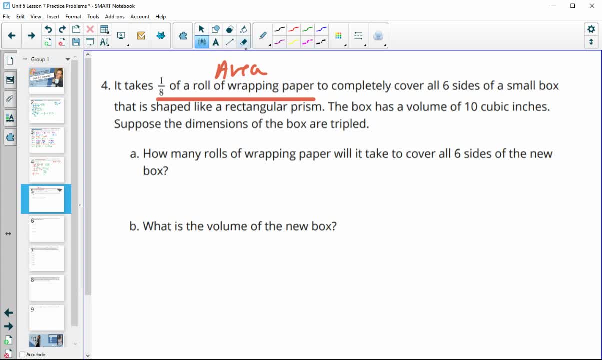 takes to cover it. The box has a volume of 8. And then we have a volume of 8. And then we have a volume of 10 cubic inches. Okay, so its volume is 10 cubic inches. Suppose that the dimensions 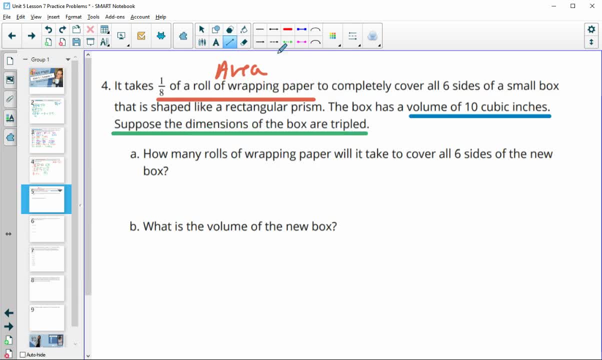 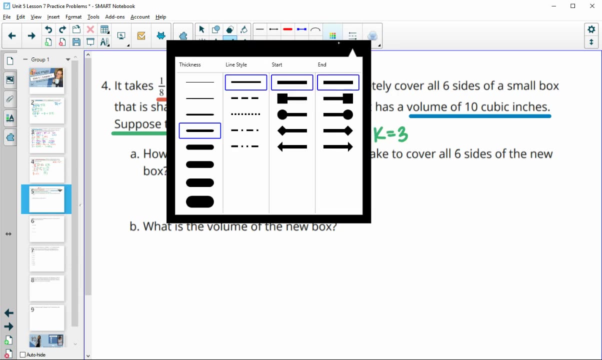 are tripled, So they're giving you a scale factor here. So when we triple the sides, that gives us a K value of three or a scale factor of three. So how many rolls of wrapping paper is it going to take now to cover all six sides? And the wrapping paper is that area? 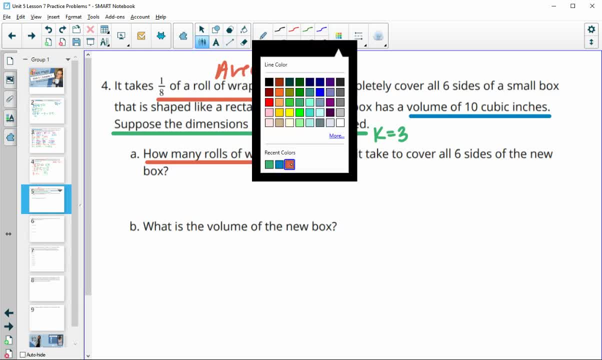 So when we're talking area, then we want to do the original area And then we want to multiply that by the scale factor squared when we're talking area. So we're going to do one eighth times three squared, So that's really one eighth times nine. So we're going to get nine eighths of. 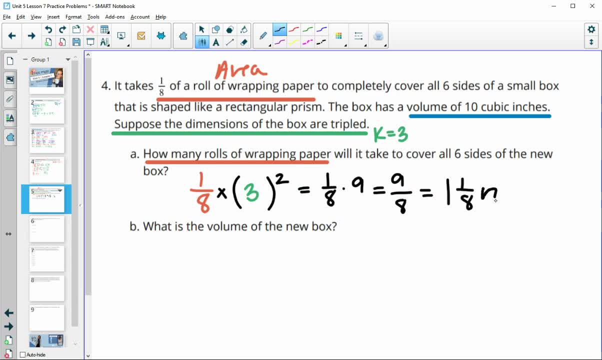 a roll, which is one and one eighths roll of wrapping paper to cover the new dimensions, And then what's the volume of the new box. So if the original volume was 10, then we will multiply that by our scale factor cubed, because when we're working in volume it multiplies by the 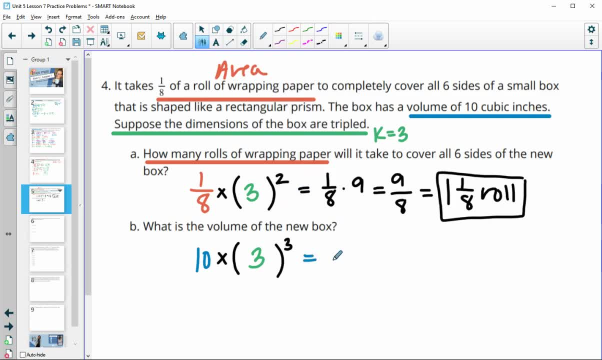 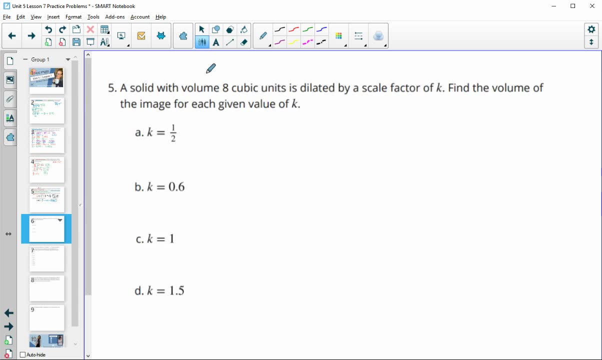 scale factor cubed. So then, our new volume is going to be 10 times 27,, or 270 inches cubed. Number five, a solid, with a volume of eight cubic units, So we're in volume, for this one is dilated by a scale factor of K. Find the volume of the new image for the given Ks below: 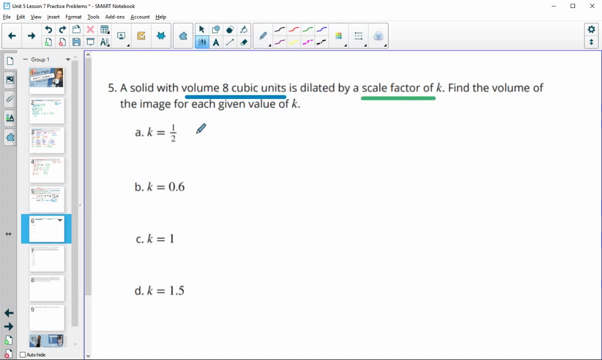 All right, so we've got our original volume and then we will just be multiplying this original volume. So I'm going to take the original volume and write it down for each one, And we're going to take our new volume times the scale factor cubed, since we're in volume. So we'll be wanting. 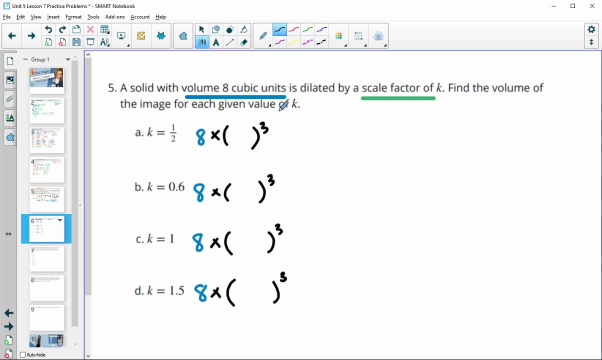 to take scale factor cubed each time and that will give us our new volume. So in this case it was times one half. In this time it was times 0.6 cubed, times one cubed and times 1.5 cubed. 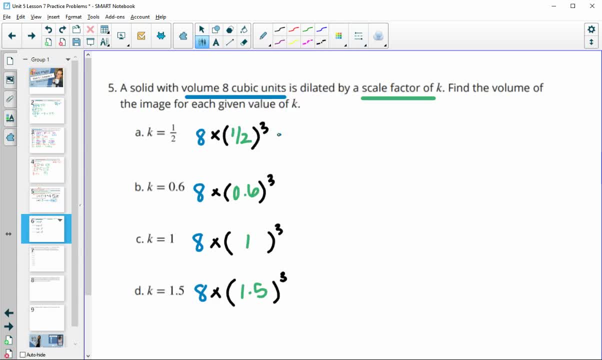 So when we do eight times one half cubed, we'll end up with one unit cubed. our new volume, Eight times 0.6 cubed, is going to give us 1.728 units cubed. Eight times one cubed will just give us eight units cubed. 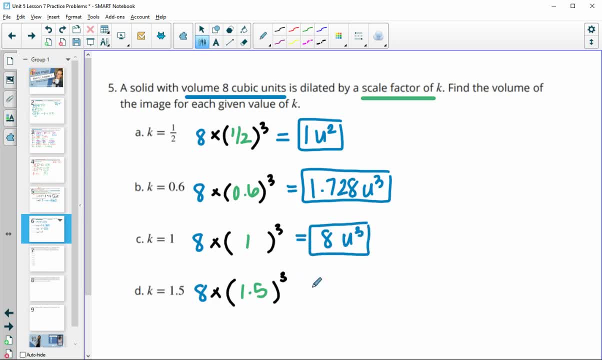 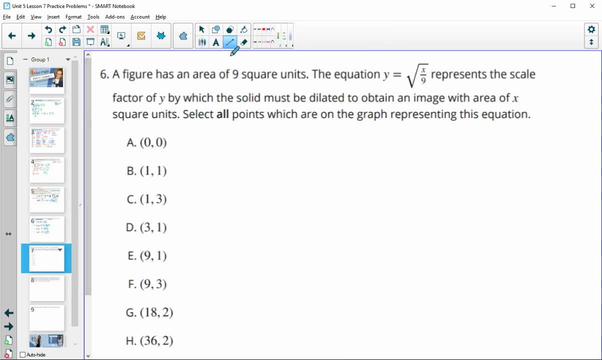 because that one won't change at all. And then eight times 1.5 cubed will give us 27 units cubed for that new volume. Next one: a figure has an area of nine square units, So we're talking area here. Then it gives. 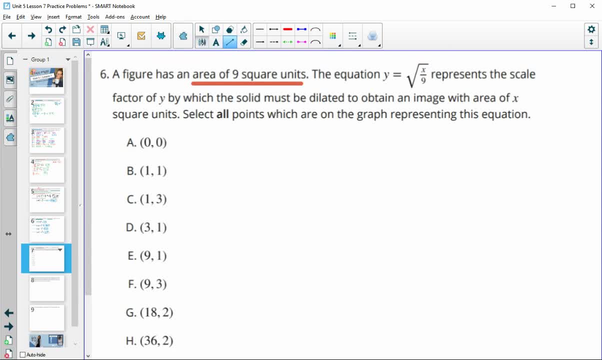 us this equation that represents the scale factor of y, for which the solid must be dilated, And so we're just going to plug all of these points in to see which ones are on the graph. So remember, the first one is x, the second one is y, So we're going to plug in the x. 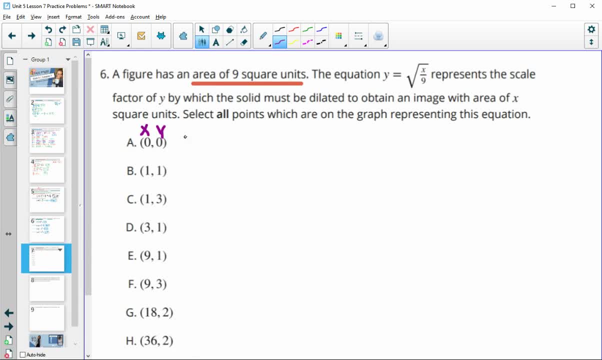 and see if they equal the y value. So for this one we've got square root of 0 divided by 9, and 0 divided by 9 is 0. And then the square root of 0 is 0. So we plugged in 0, we got back 0.. 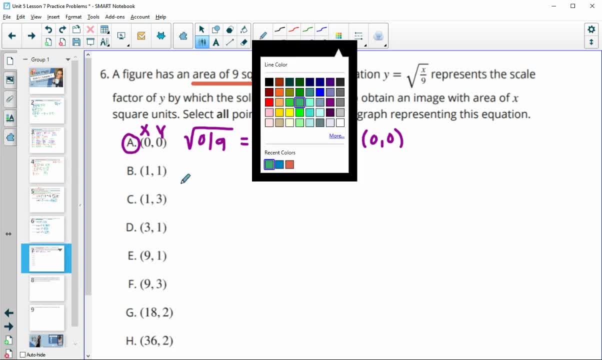 So this one is good. Second one: we are plugging in 1, and we're hoping to get back 1.. While the square root of 1 ninth is not going to give us 1,, it's going to give us 1 third. 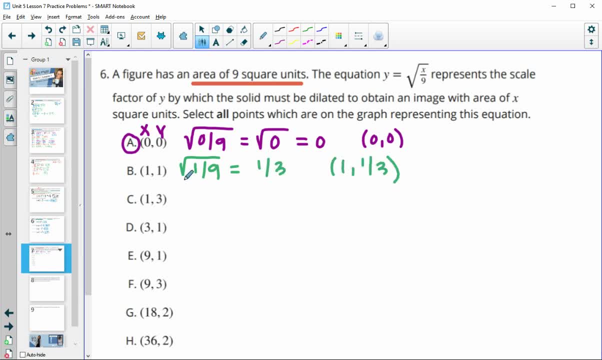 So this one we plug in 1, and we get back 1 third. So this one would be wrong. That also tells us this one is wrong because we know when we put in 1, we get back 1 third. So we can cross that. 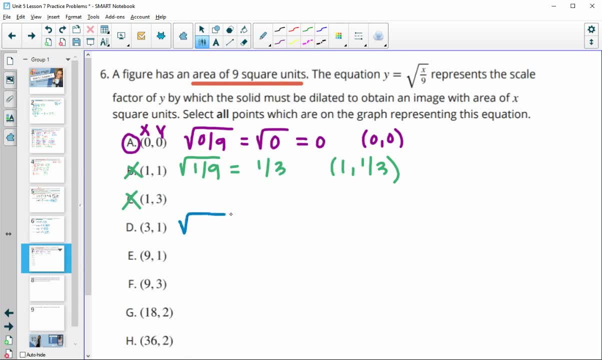 one out right away. This one, we're going to plug in 3.. So we're going to do 3 divided by 9. And 3 divided by 9 is 1 third, And then the square root of that isn't going to be nice. 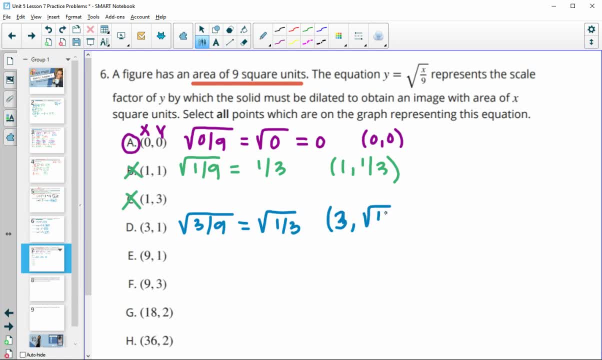 So when we plug in 3, we get back 1 third. So this one we plug in 1, and we're hoping to get back the square root of one third. So this is not good, or is not on our graph E. we're going to do nine. 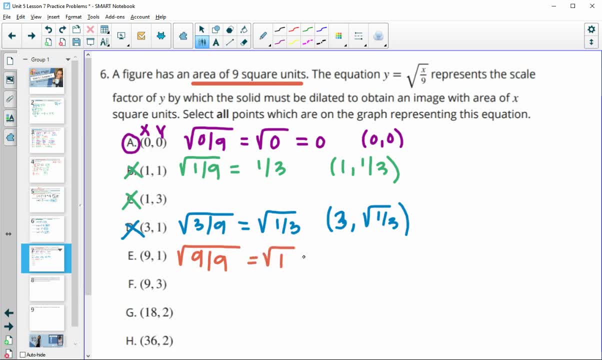 divided by nine, and nine divided by nine is one and the square root of one is one. So when we plug in nine, we get back one, which is this point, which means this one cannot be there, because if we plug in nine, we get one, not three, And then the next one we're going to plug in 18.. So we'll. 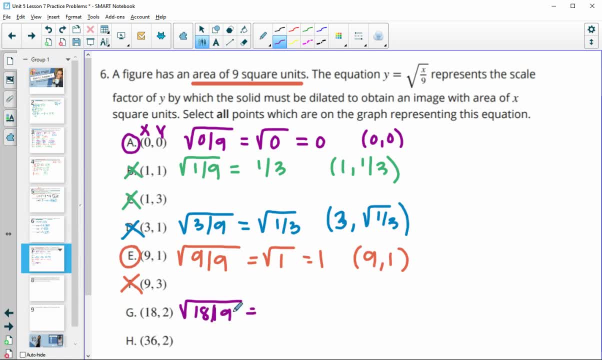 have 18 divided by nine, and 18 divided by nine is two. So when we plug in 18, we get back the square root of two. So not this. And then the final one in this will be 36 that we'll plug in. So we'll do. 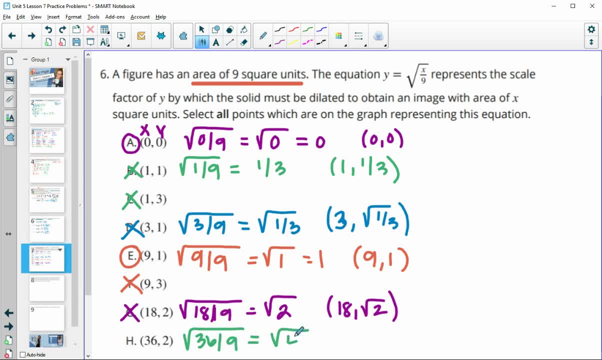 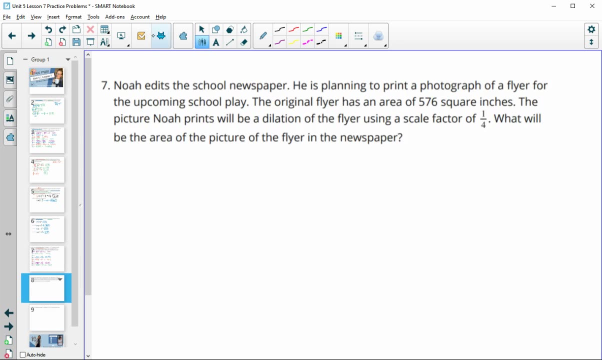 36 divided by nine, and 36 divided by nine is four, and the square root of four is two. So when we plug in 36, we get back two, which is this point, So that one's good. Number seven, Noah, edits the school newspaper. He's planning to print a photograph of a flyer for 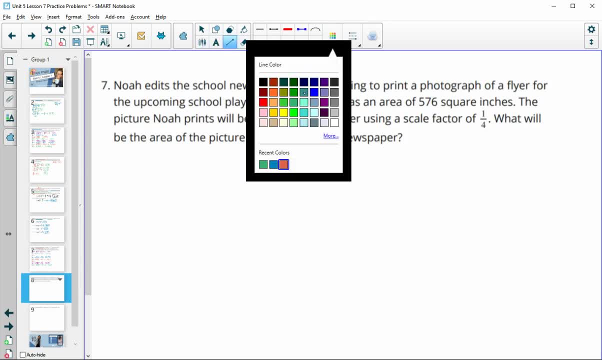 the upcoming school play. The original flyer has an area of 576 inches squared. The picture Noah prints will be a dilation of the flyer using a scale factor of one fourth, What will the area of the new picture be? So remember, for when we're talking, areas we'll take. 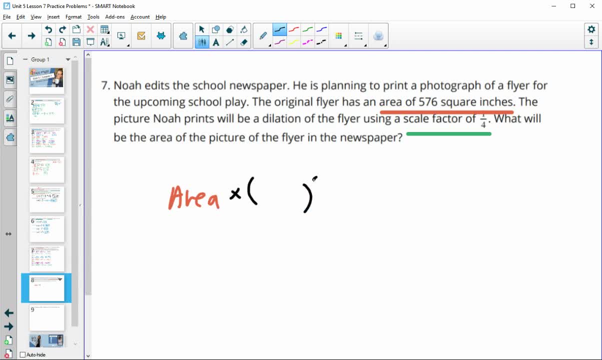 the area and then we'll multiply it by the scale factor squared, And then that will give us our new area. So the original flyer area is 576 square inches, And then we're going to multiply that by one fourth squared, And when we do that we will get a new area of 36.